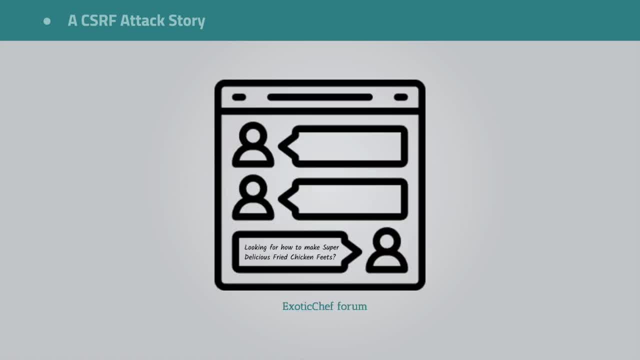 You search and search and you finally find this comment on the exotic chef forum Looking for how to make super delicious fried chicken feets. Get the recipe here. You click the link and after a moment this message appears. You laugh and decide to stop your meaningful quest. However, if you knew what really happened, 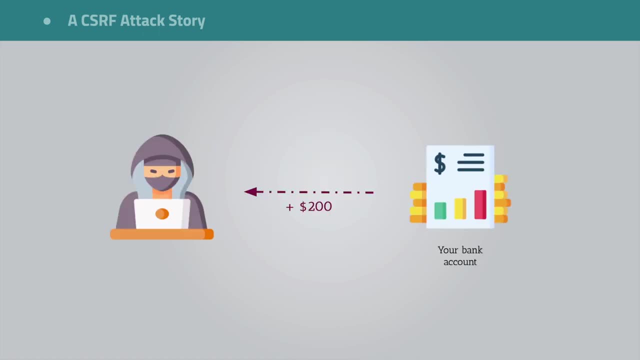 you wouldn't laugh, believe me. The trickster who made you laugh treated himself to $200 from your bank account. Wait, wait, what? How did they do that? Well, here's what happened. The joker found out that the money transfer platform you're using uses the get method for. 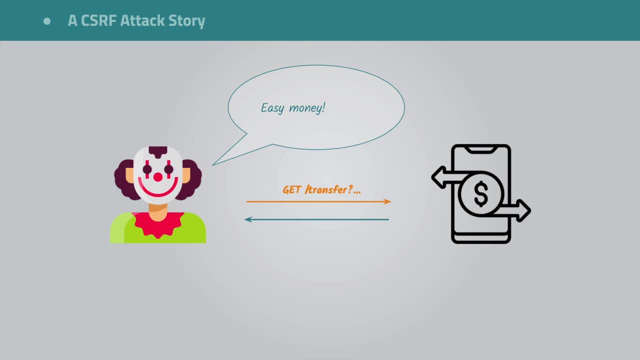 important actions such as transfer funds, which is a very insecure way to make transfers or any sensitive action for that matter. So you click the link and after a moment this message appears. You laugh and decide to stop your meaningful quest. However, if you knew what really happened? you'd laugh and decide to stop your meaningful quest. However, if you knew what really happened, you'd laugh and decide to stop your meaningful quest. So you click the link and after a moment you'll see that the money transfer platform you're using uses the get method for important actions. 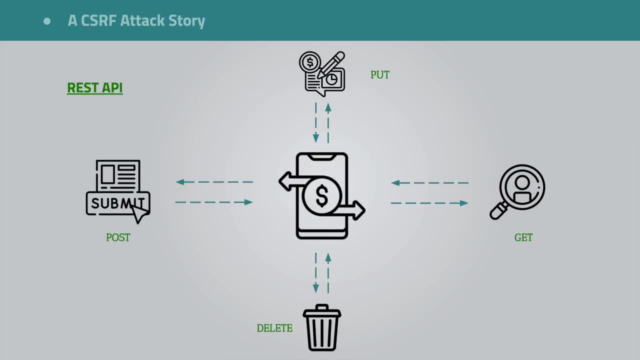 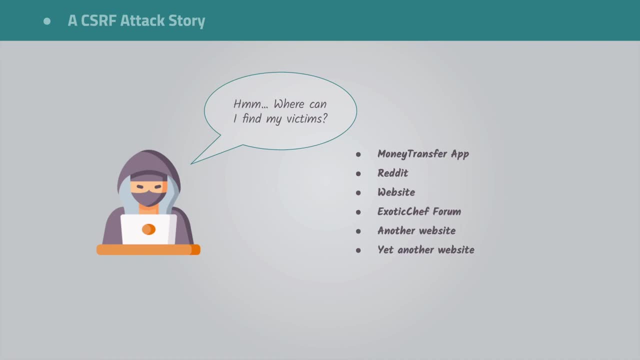 such as transfer funds or any sensitive action for that matter. Had the app followed the rest approach, such actions would have been performed using post requests, which is a better and safer way. Anyway, as a second step, the hacker tried to list websites and ways to find money transfer. 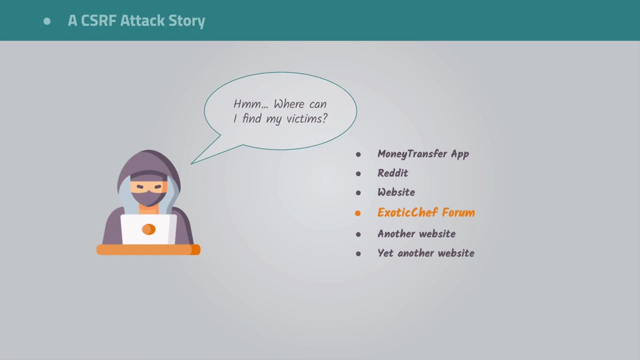 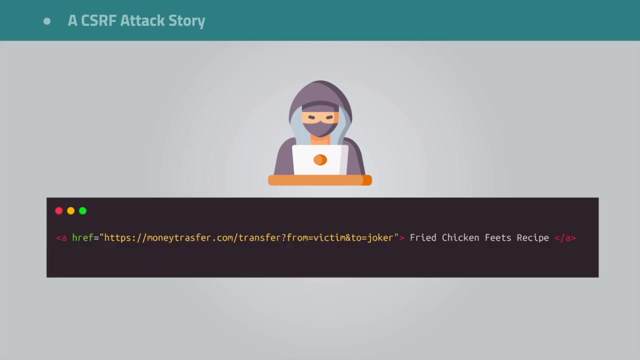 clients. Apparently, the exotic chef forum was on the list, which is weird, but you got the idea. The third step the attacker would perform is crafting malicious requests to transfer funds from victims like you to the hacker's account. So the link the attacker crafted would take advantage. 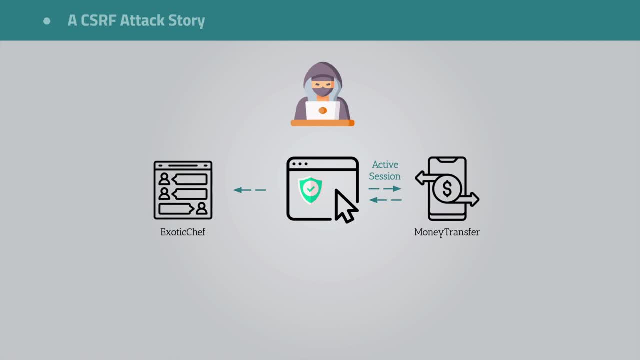 of you being locked in to the platform and trigger the request, because the browser assumes that's you making the request, or at least you know what's happening- and boom. Well, actually $200 is not a big deal, but, believe me, if the transfer proved to be successful, the joker will do it again. 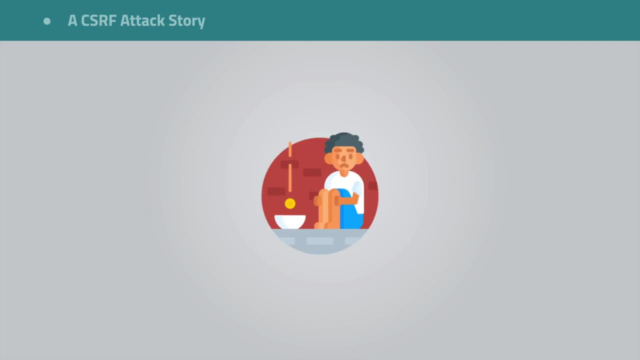 and the second time you'll end up living in the street. A C-Surf attack is a way to take advantage of the trust relationship between the browser and an API or a website and then leverage that to forge requests to stop the hacker from doing the same thing. This is a way to take advantage of the trust. relationship between the browser and an API or a website and then leverage that to forge requests to stop the hacker from doing the same thing. This is a way to take advantage of the trust relationship to stop the hacker from doing the same thing. This is a way to take advantage of the trust method. 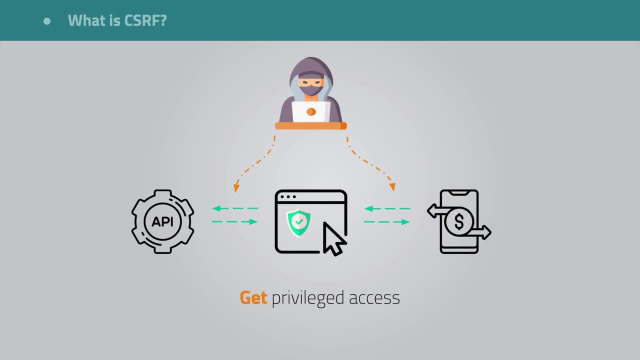 to stop the hacker from doing the same thing. This is a way to take advantage of the trust method to stop the hacker from doing the same thing. Div, pass another a bug, mac, by just saying you're Catnee Diospeed and emite this. 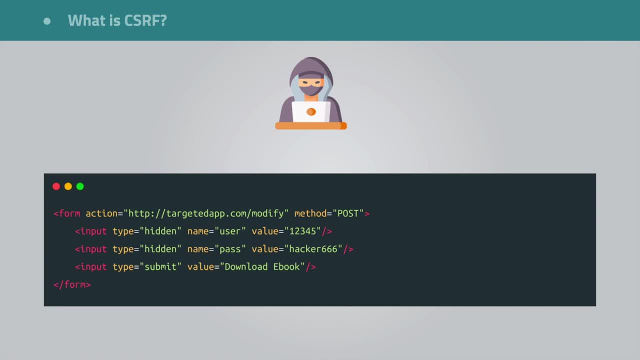 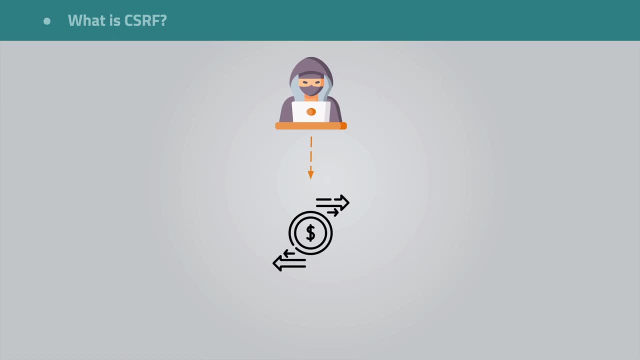 line or form to induce users to perform actions they do not intend to perform. Examples of such actions are password reset, funds transfer or, as we've said, if the user is an admin or has lots of privileges, the attacker could actually gain full control over the system, Usually a C-Surf. 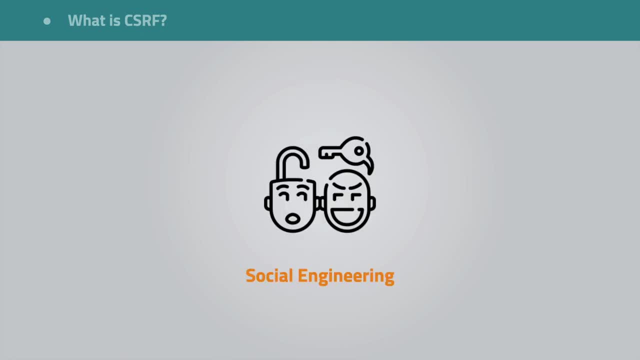 A C-Surf attack is possible with a little bit of social engineering and crafting tricky ways to trigger the request, such as malicious links, fake forms and even invisible resources such as a picture with the malicious link in the source field, And fortunately, most of the time the request goes unnoticed by the victim. 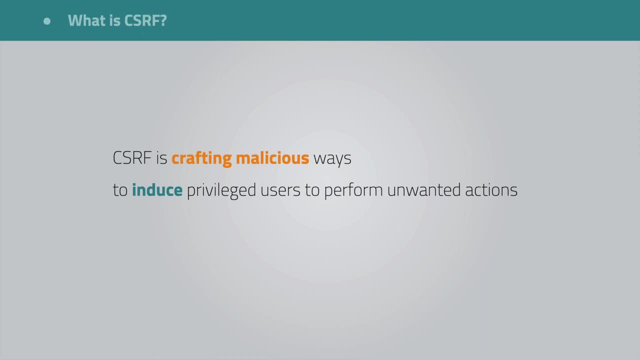 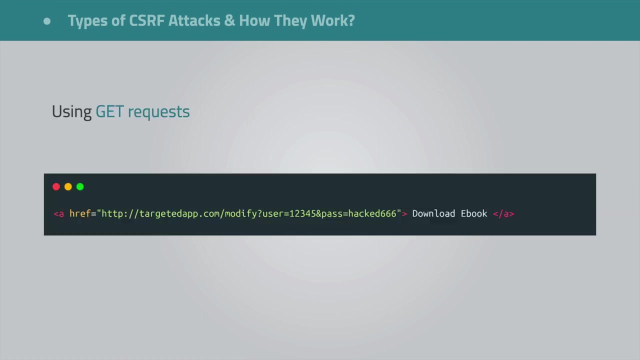 So a C-Surf attack is a method to induce privileged users to perform unwanted actions, And the target is functionality that causes a state change on the server. Great, now let's zoom in a little bit and see that in action. From the previous story, we know that a crafted, malicious GET request is one way to perform. 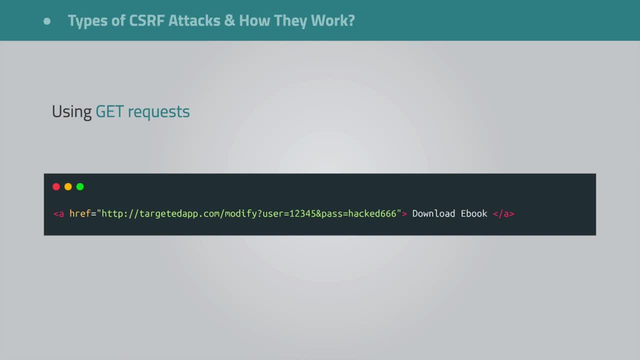 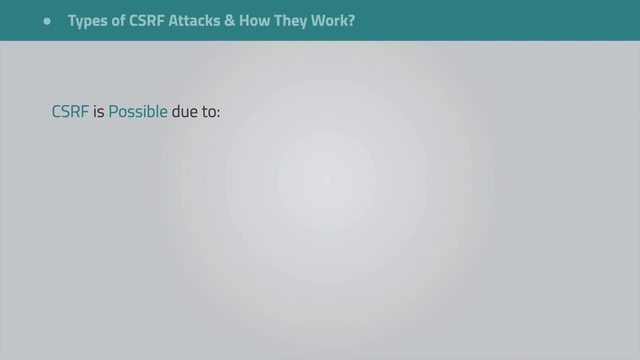 a C-Surf attack. This is one of the most basic and common forms of C-Surf attacks. Before we dive into what happens, it's important to know that vulnerabilities to C-Surf attacks are caused by state change in actions that are performed using insecure methods, wherein 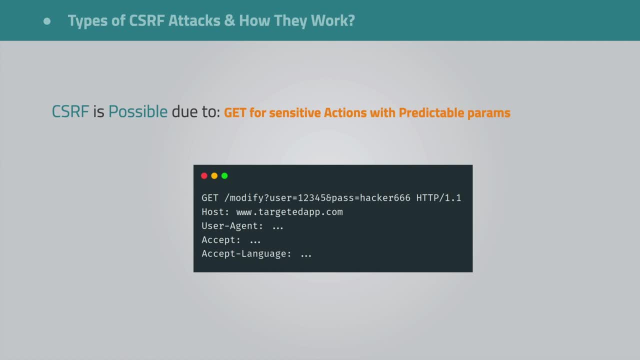 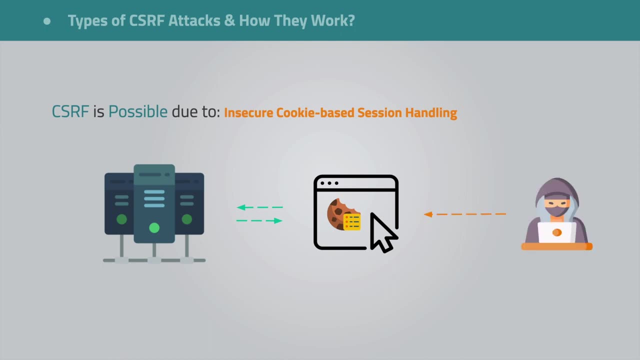 request parameters could easily be predicted by attackers. Also, cookie-based session handling Without any other mechanism to validate requests is an inviting opportunity to a C-Surf attack, And that's because the browser sends session cookies with every request sent from your browser. 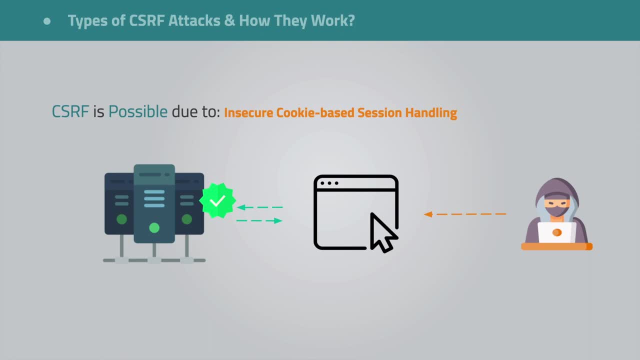 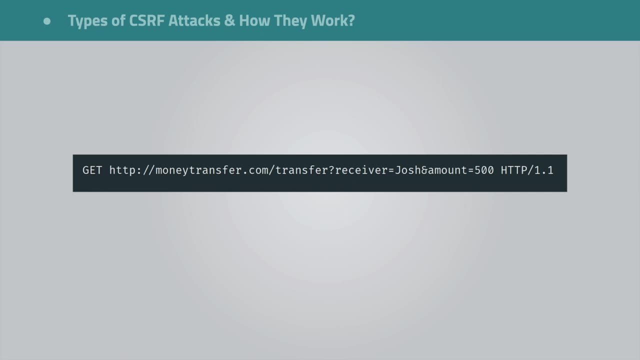 So there is no way the browser will detect that a request is forced. So here's how it happens. If the fonts transfer could be performed through a GET request like this, then a C-Surf attack is easy. The attacker could craft an email with HTML content and include this line, for example: 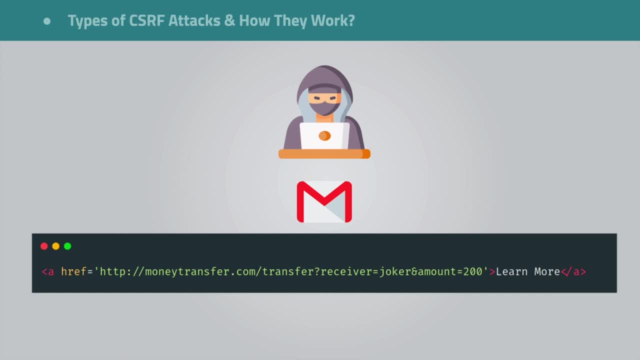 And because you're curious about how to make a C-Surf attack. the attacker could craft an email with HTML content and include this line, for example: If you want to make a delicious plate full of fried chicken feeds, you won't hesitate to click the link to learn more about it. 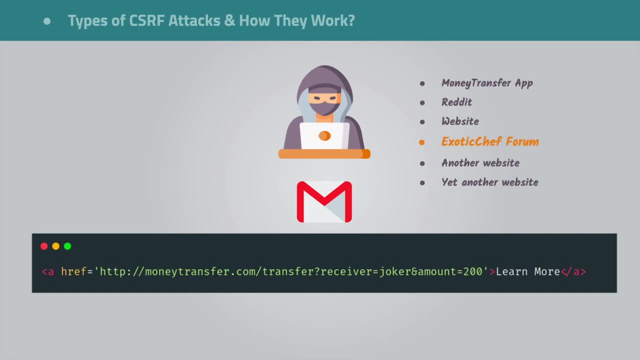 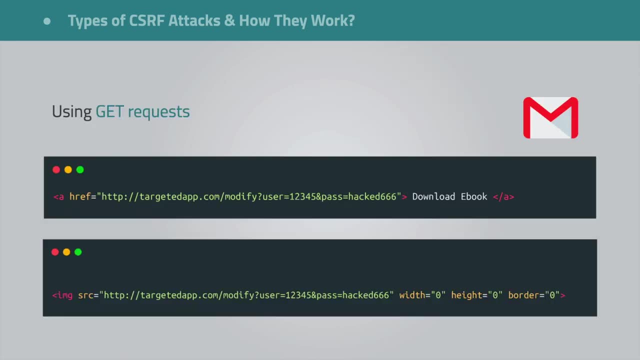 The link could also be in a website that the attackers know you're more likely to visit, and with a little bit of social engineering, you end up eating out of the trash. So this is how a C-Surf attack is performed using a GET request. 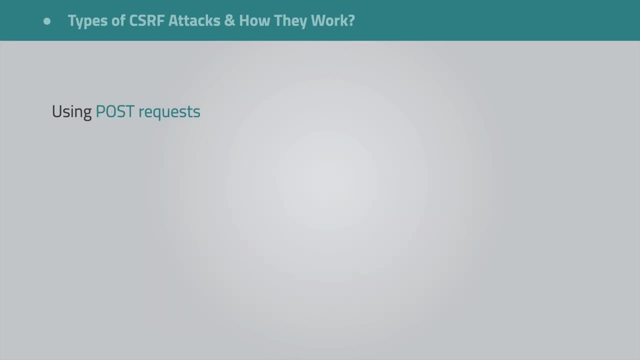 Let's see now a POST request example. When sensitive actions are performed via POST requests, the attacker cannot use single links via the A tag or an image or any similar way, And this is how a C-Surf attack is performed using a GET request. 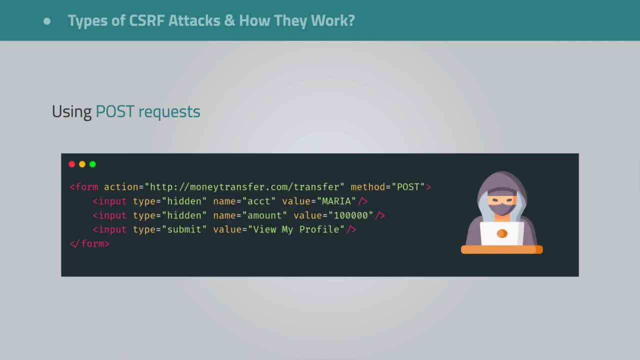 The way to forward a request here is to use a form that will be submitted by the user or automatically. In this example, the attacker crafted a form that contains the parameters needed to make the transfer, but they are hidden. The user won't know what is happening here. 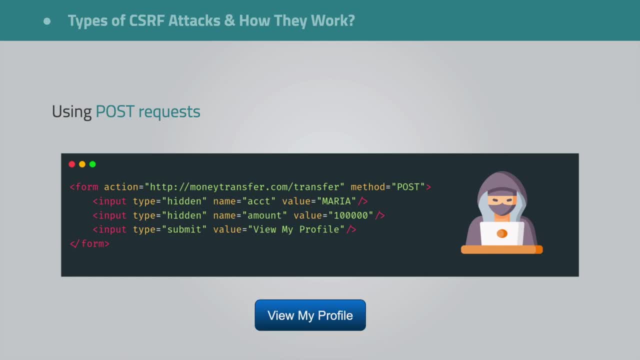 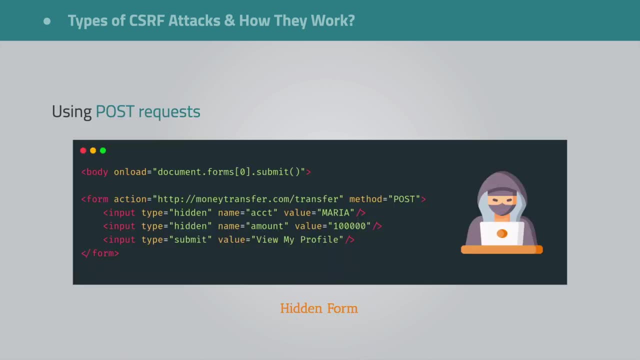 They even may be unaware it's a form. The button will contain something inducing for the user to click, And voila, the transfer is done, And sometimes the form could be invisible and gets submitted automatically using JavaScript. Alright, And one very important note before we talk about how to protect ourselves from a C-Surf: 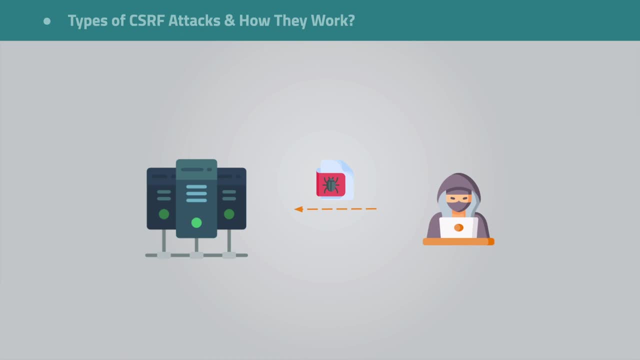 attack is that it is possible for such attacks to be stored on the website itself. If the vulnerable website accepts user input that allows raw HTML, the user could send the malicious link as an image tag or iframe to the backend of the website, And this increases the likelihood to get the victim. 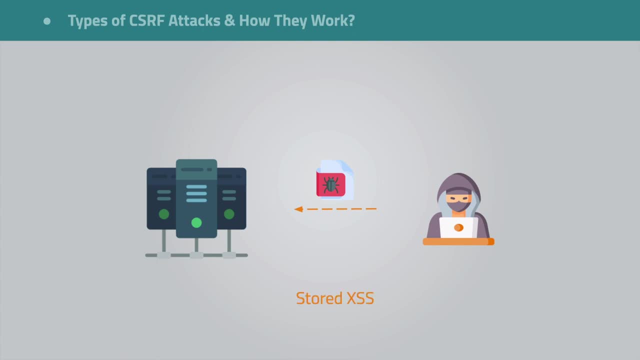 This is achieved through a stored cross-site scripting attack, which is explained in the previous video in more detail, And, as you might have guessed, this type of attack is called the stored C-Surf attack Sweet. So we've seen how a C-Surf attack is usually performed. 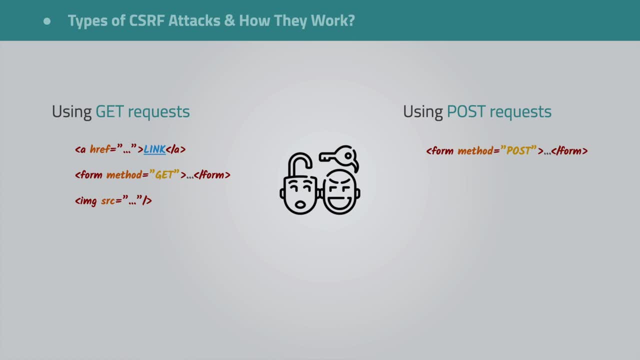 The attacker could find other ways to do this, but basically it's one form or another of what we've seen. Now, if you are wondering how to defend against a C-Surf attack, then keep watching. Well, first thing to make sure is that sensitive actions cannot be performed using GET requests. 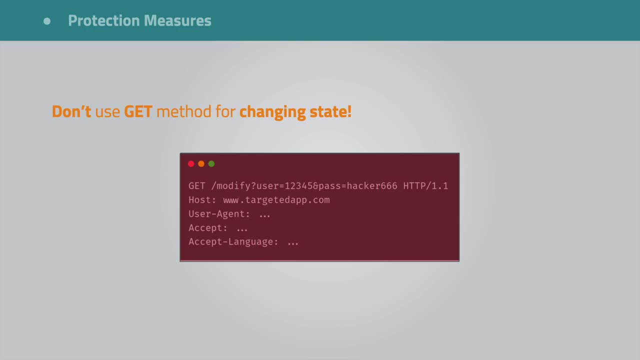 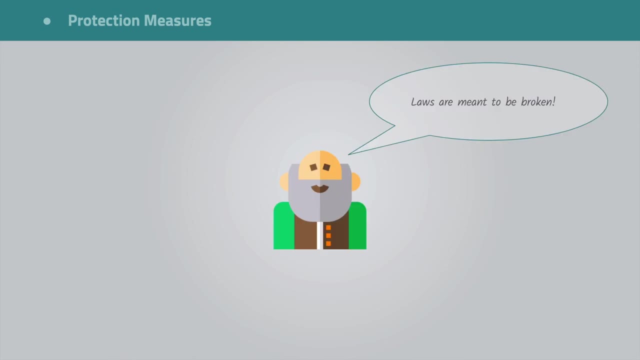 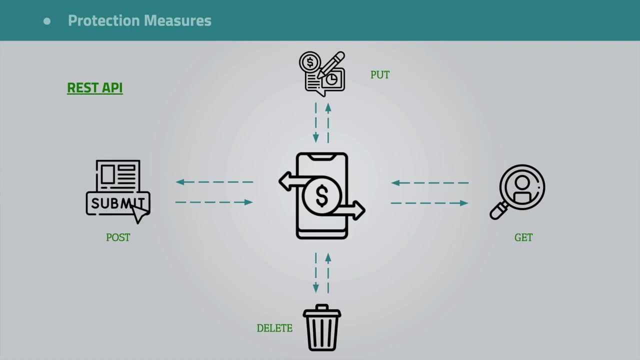 That would be an easy cake for the hacker. It's a very basic thing: Follow REST principles. And speaking of principles, I'm certainly sure whoever originated the famous saying that laws are meant to be broken doesn't know REST. REST encourages developers to map API actions to the appropriate HTTP verb. 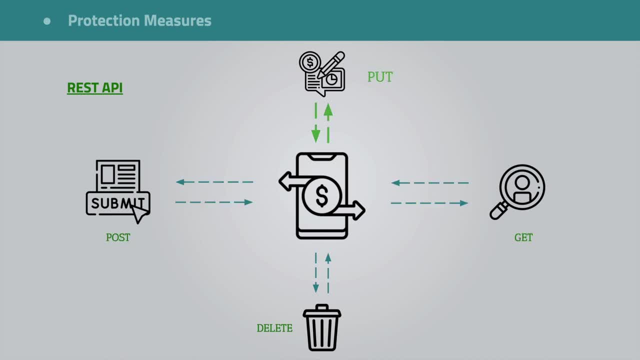 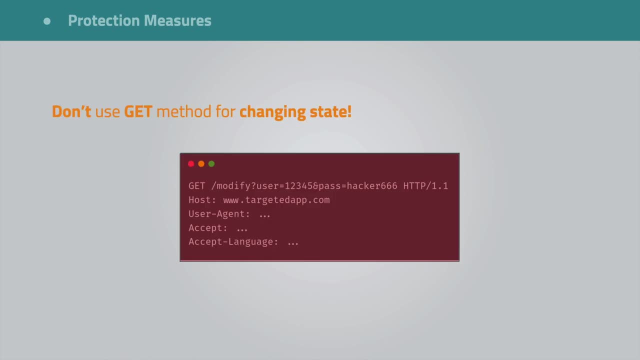 Use GET for fetching POST, for modifying PUT, for adding new objects, etc. Changing the state of the server using the GET method is very unsafe. Okay, great, Now we're at least sure the hacker won't find it easy. Let's make it easy to C-Surf us or our users.